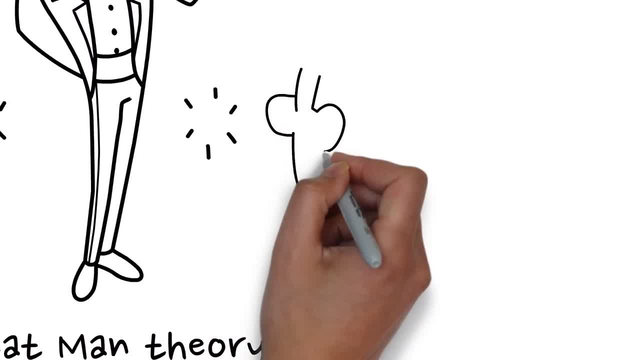 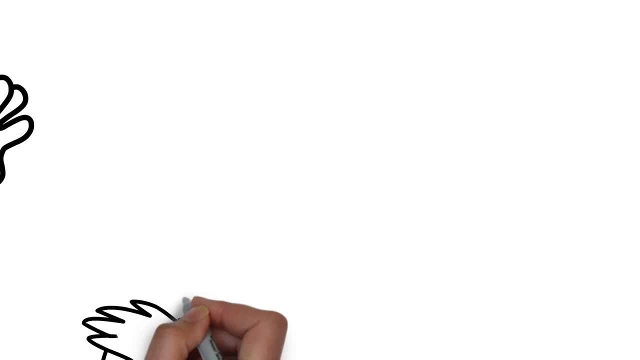 made has largely been refuted. The main importance of this theory is that it reveals how we have traditionally seen leaders. Carlyle's work also gave impetus to the study of leadership and development of further leadership theories: Control and domination, power and influence. 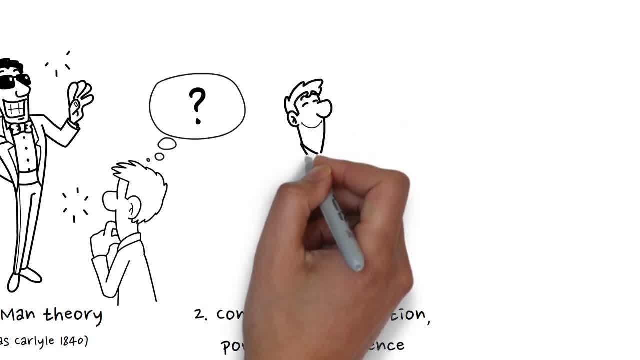 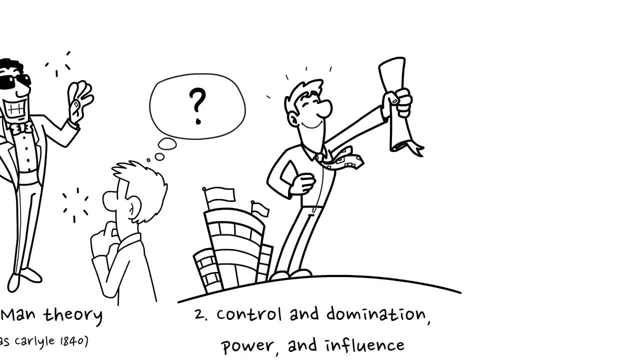 Great man theory was linked to the idea of power and that leaders would naturally dominate others by the strength of their personality. This school of leadership theory is summed up in Moore's definition of leadership from 1927. He defined leadership as the ability to impress the 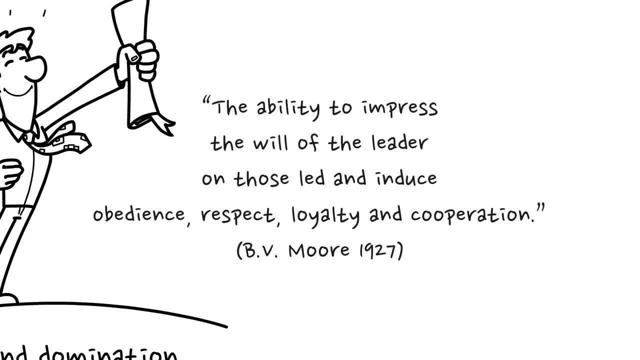 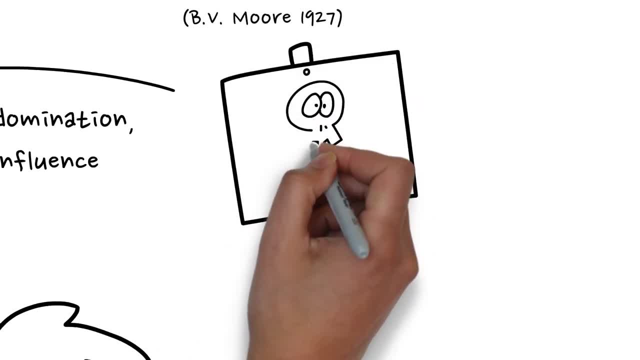 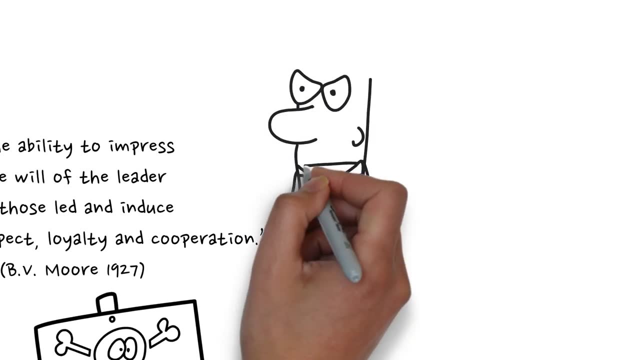 will of the leader on those led and induce obedience, respect, loyalty and cooperation. The point to note here is that there is no reference to the responsibility of a leader for their followers or to any moral code. It took the extreme abuses of power by the likes of Hitler. 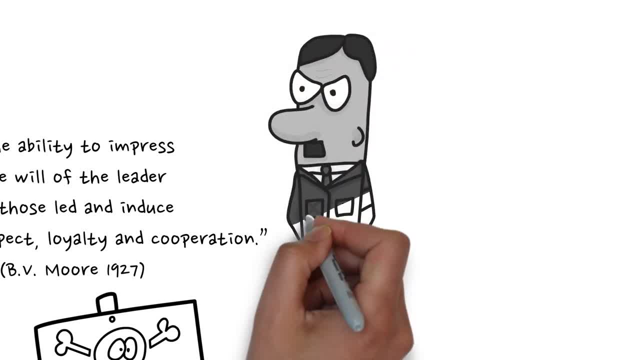 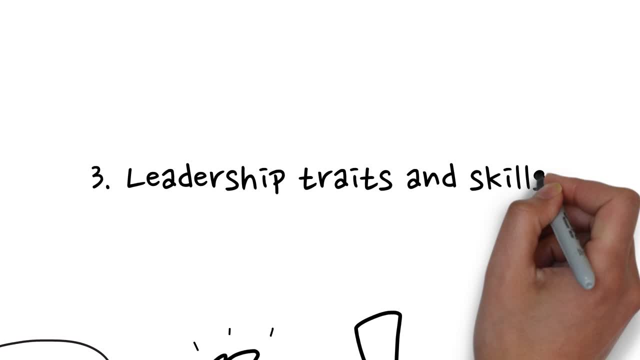 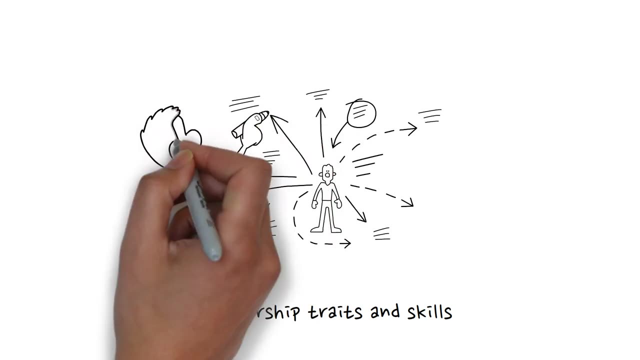 Mao and Stalin in the first half of the 20th century. for these ideas of leadership to be properly challenged- Leadership traits and skills. Academics also started to identify the traits of leaders to see what common characteristics made a good leader In the early iterations of the theory. 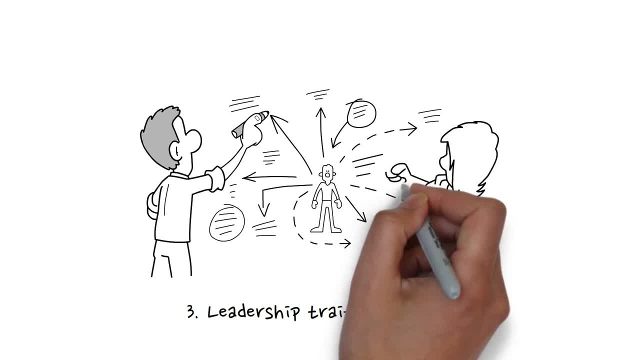 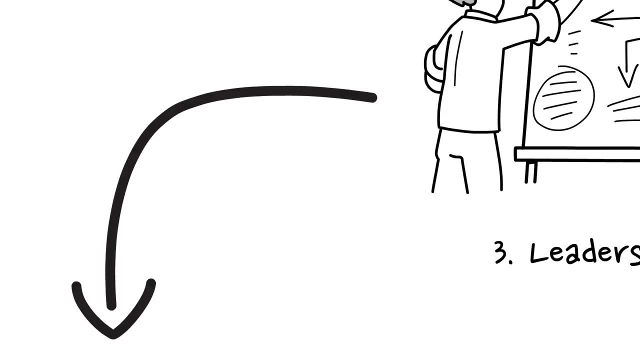 these traits were also seen as inherited and linked to the idea of the great man, the charismatic male hero who was tall and good looking. This school of thinking evolved into identifying more positive traits such as integrity, moral courage and humility. Importantly, 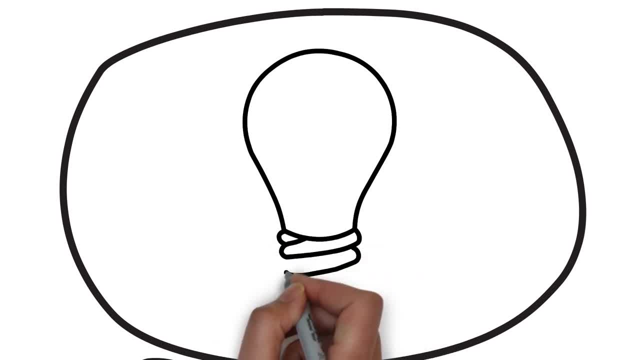 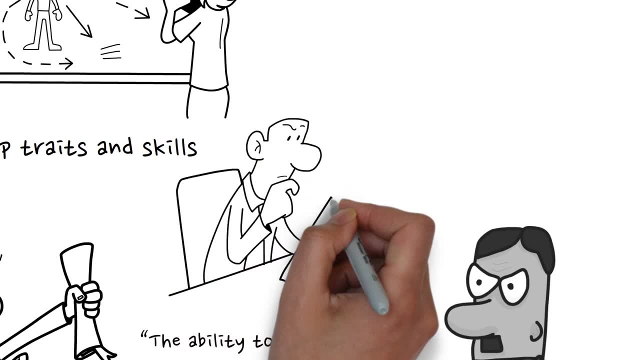 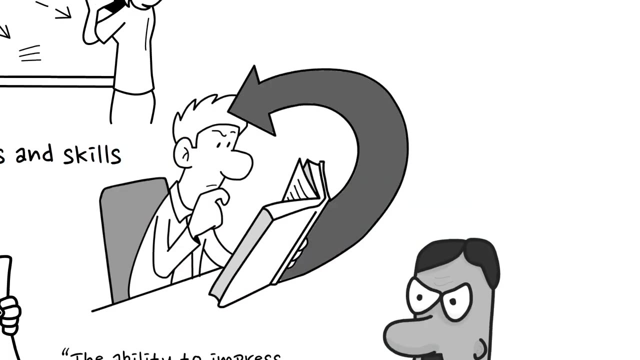 there was also a shift towards characteristics that could be developed, As the emphasis moved from innate to acquired characteristics. the focus moved to identify leadership skills and behaviours that could be learned, such as communication, strategic leadership and decision making. Action-centred leadership- John Adair's action-centred leadership model. 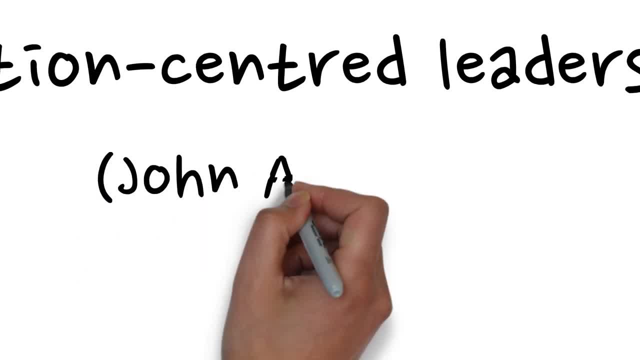 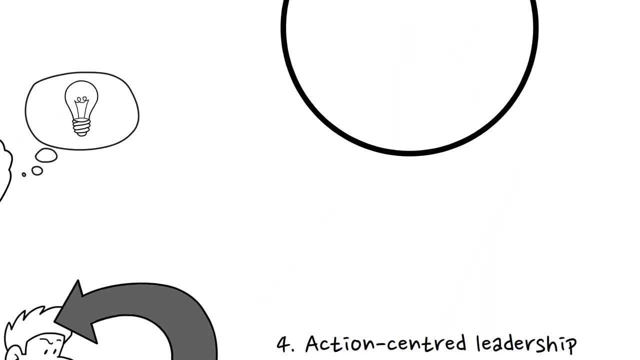 was built on the premise that leadership skills and behaviours could be taught and adopted. The simple idea behind action-centred leadership is the need to balance the three core management priorities of task, team and individual. A good leader must continually seek to achieve the task. 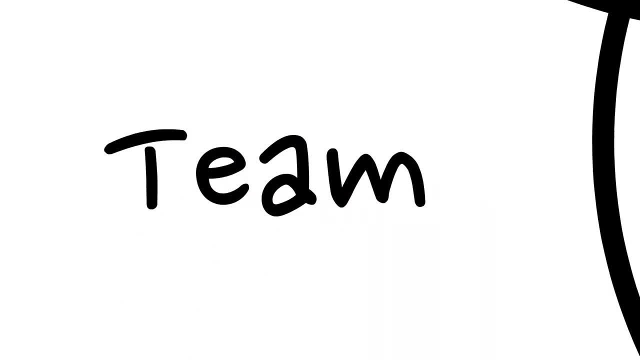 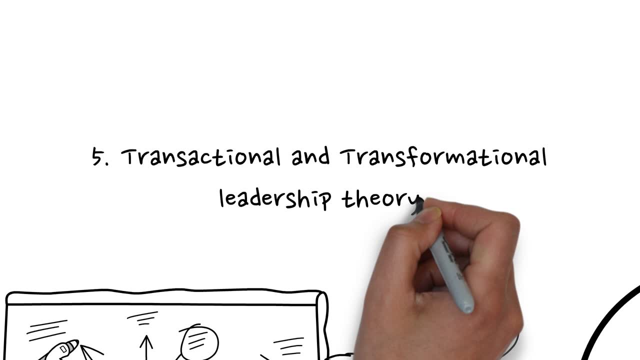 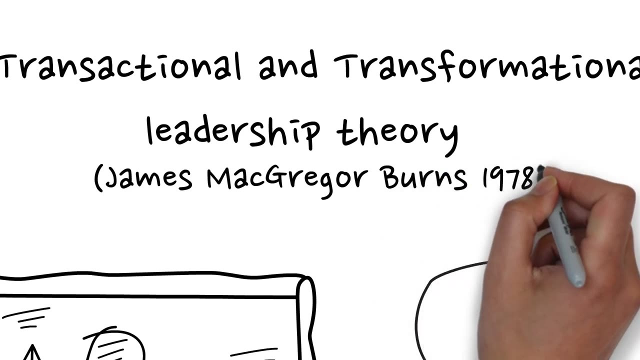 build the team and support the development of each individual Transactional and transformational leadership theories. James MacGregor Byrne took the ideas of influence and behaviour in another direction when he defined the difference between transactional and transformational leadership in 1978.. Transactional leadership is management using 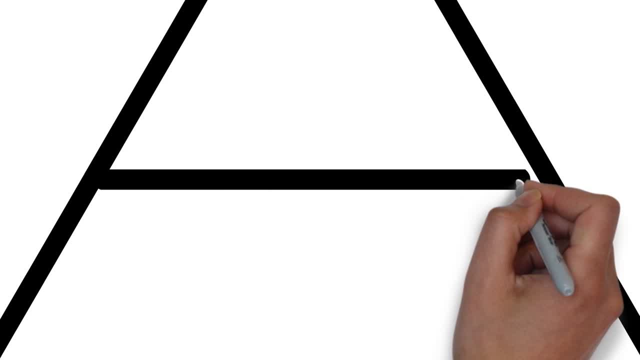 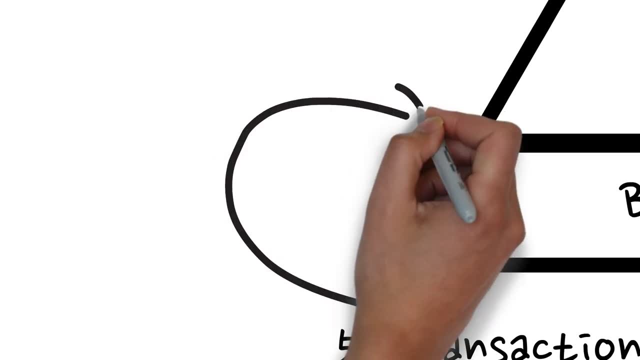 a carrot and stick approach. This functional style relies on basic human needs, such as income and job security. These elements are related to the lower end of Maslow's hierarchy, which is the hierarchy of needs. Transformational leadership goes beyond transactional leadership. 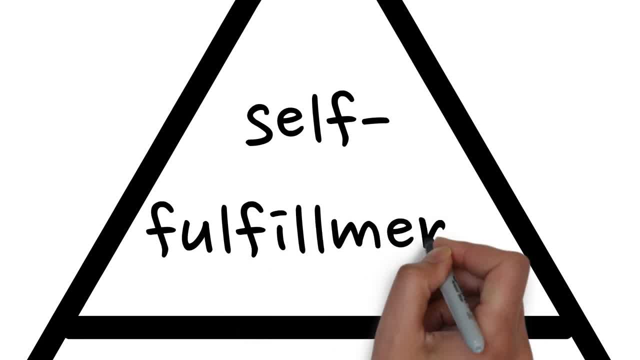 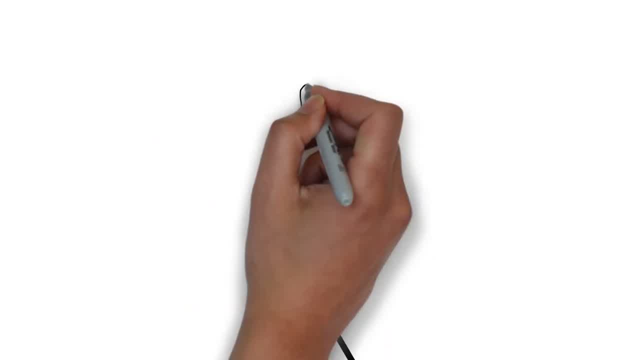 This type of leader seeks to inspire people with a compelling vision and lead them towards self-actualisation at the top of the Maslow pyramid. Bernard Bass built on the work of Burns and defined the key behaviours of the transformational leader as being a positive. 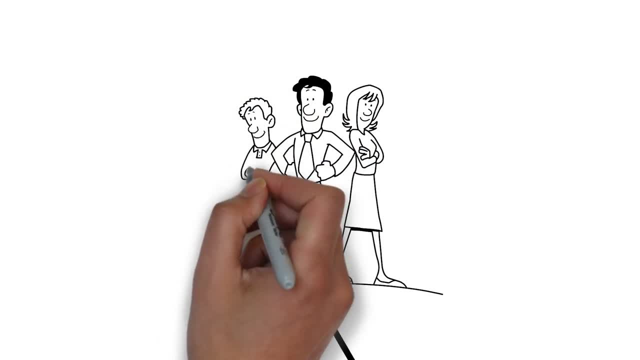 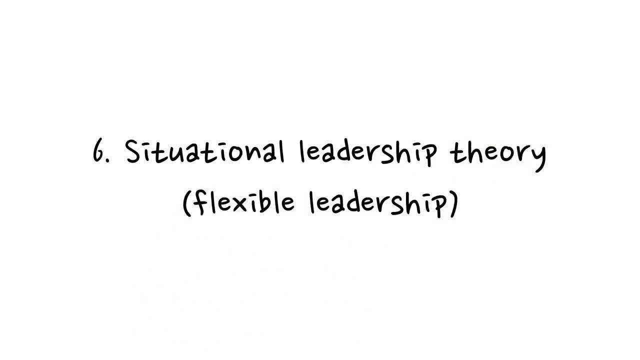 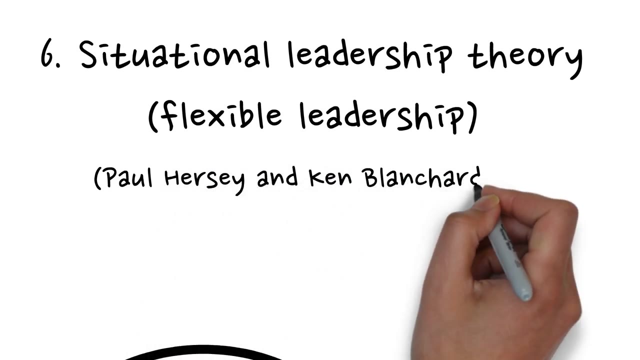 role model, providing encouragement and supporting followers to fulfil their potential. Situational leadership theory. The situational leadership model developed by Paul Hersey and Ken Blanchard took leadership theory in another, slightly different direction. Their model is about having a flexible approach. It demonstrates how a leader can adapt their management style. 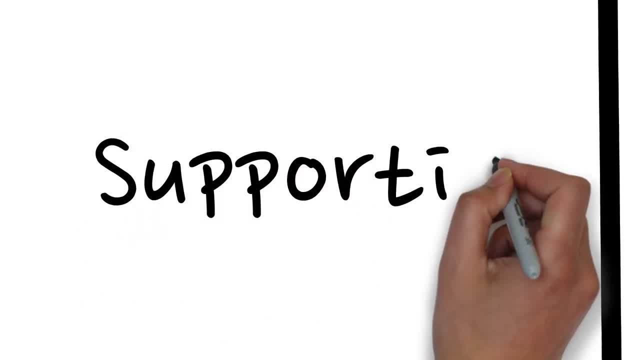 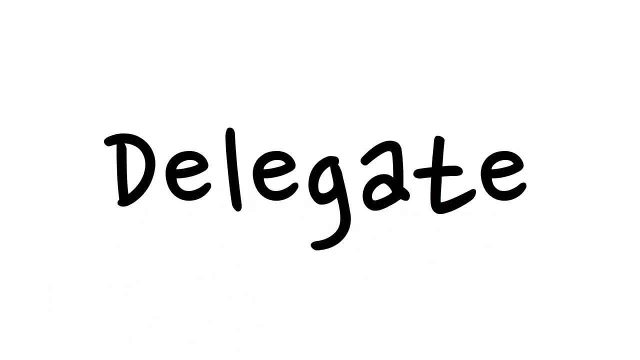 depending upon the experience of the team and the individuals they are working with, while also considering the environment and circumstances they find themselves in. The leader chooses their approach: either delegating, supporting, coaching or directing, depending upon the situation. Values-based leadership. Values-based. 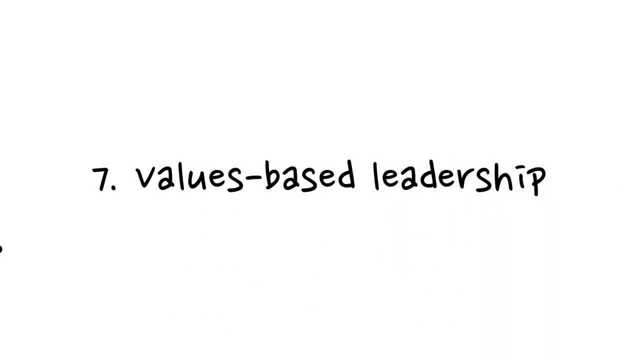 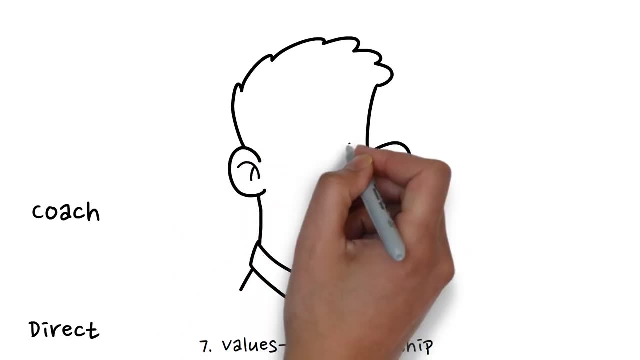 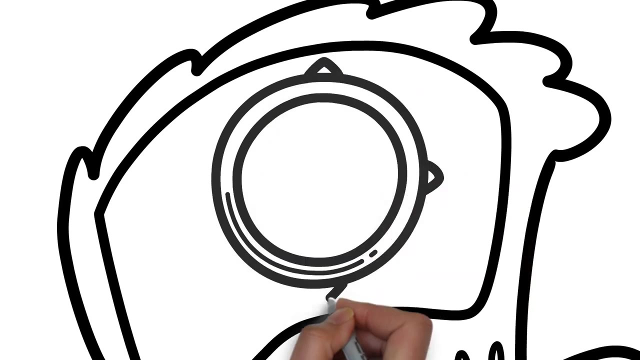 leadership developed in response to various moral failings of prominent leaders. This school of leadership, related to trait theory, encompasses both servant leadership and authentic leadership models. The central idea is that the values-based leader has a strong moral compass and leads according to their personal values and the shared values of their organisation or community. 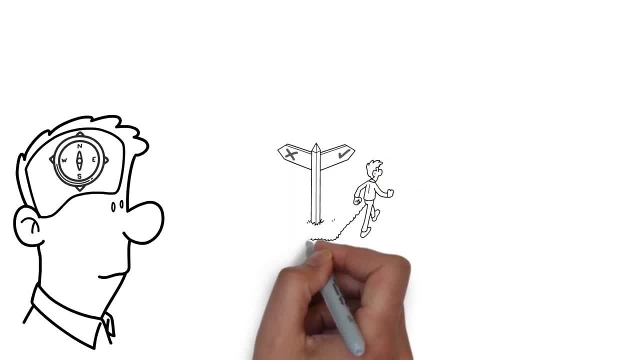 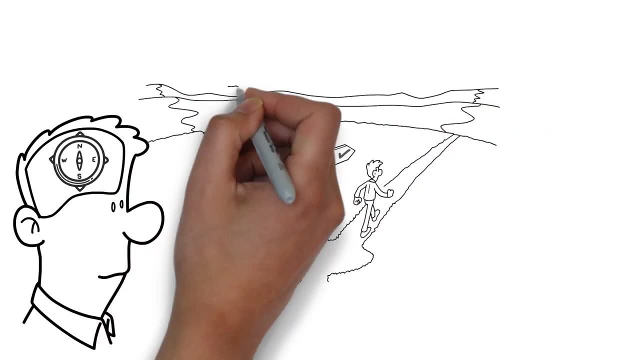 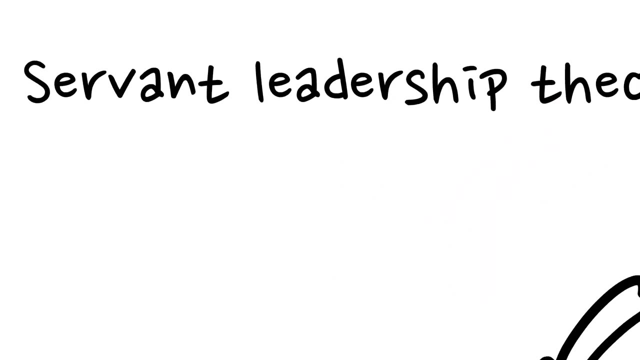 This model stresses the importance of being a good leader, not just a charismatic one, and the ability to make the right or ethical decisions, not just effective or bold choices. Servant leadership theory: The idea of the servant as leader, was developed by Robert Greenleaf. 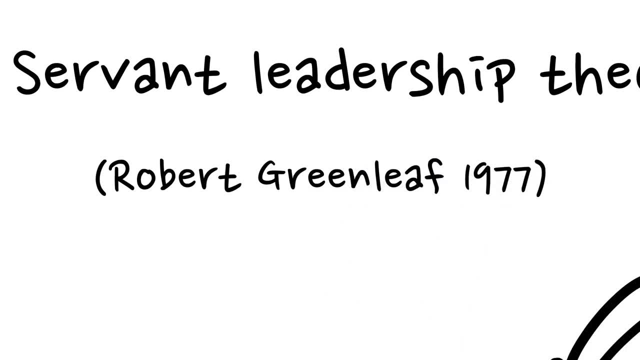 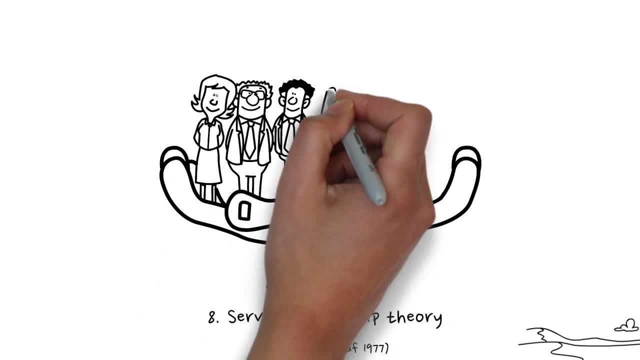 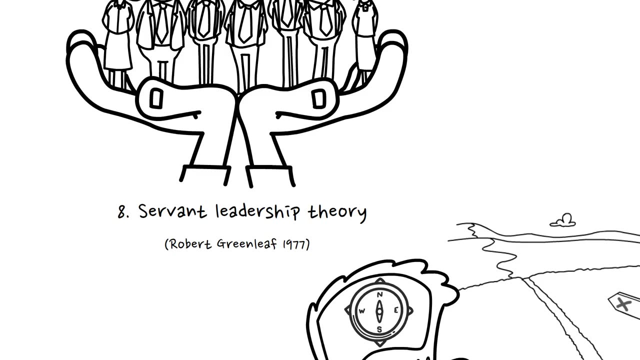 This model of servant leadership is primarily about motivation. The servant leader wants to serve others and society by raising up new leaders and helping people to move towards a positive vision of the future. They are not seeking power for themselves. Instead, servant leaders share power and empower others. Toxic or bad leaders At the other end of the scale- academics also. 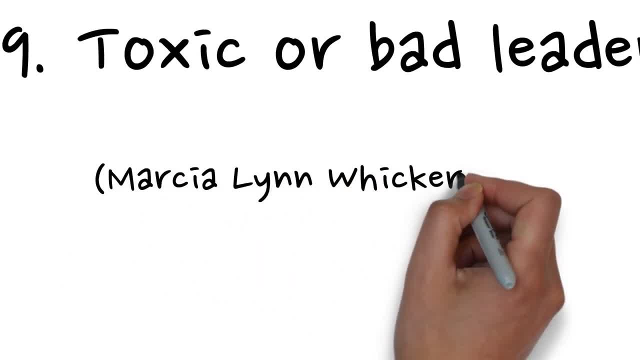 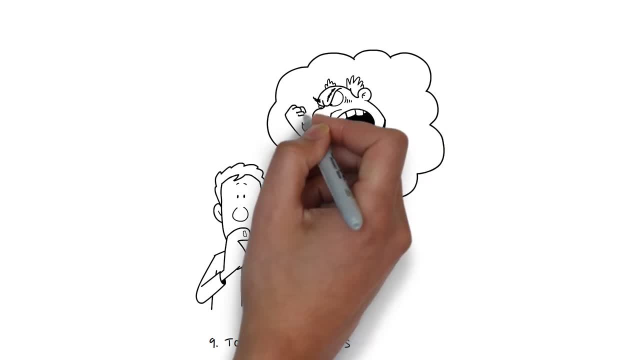 started to identify the opposite of values-based or good leaders. Marcia Lynn Wicker popularised the term toxic leader, and various models have been developed to identify such bad leadership. For example, Barbara Kellerman's study identified seven types of bad leader. 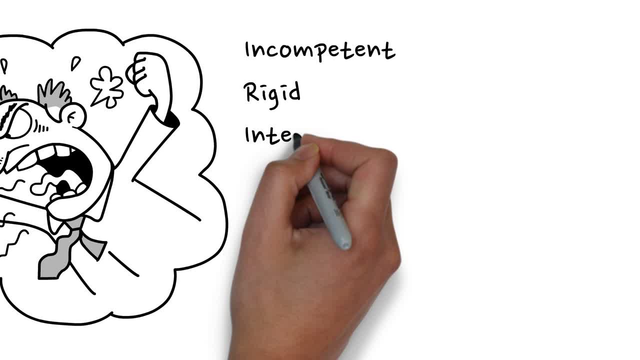 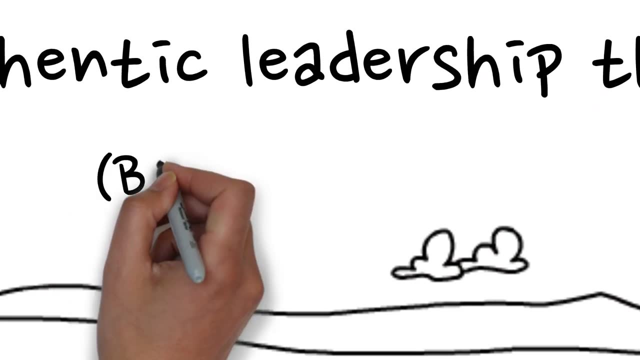 These are incompetent, rigid, intemperate, callous, corrupt, insular or evil. Authentic leadership theory- The term authentic leadership was first popularised by leadership practitioner Bill George. He wrote a book by the same name in response to failures of senior 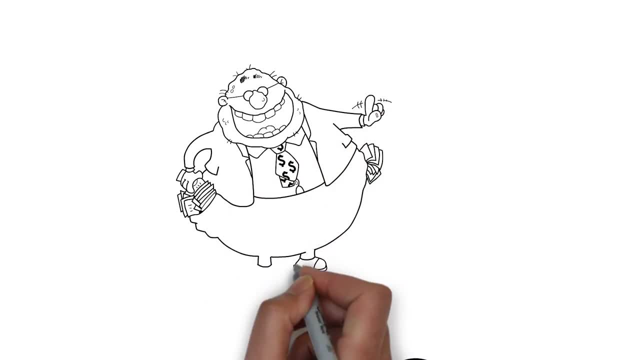 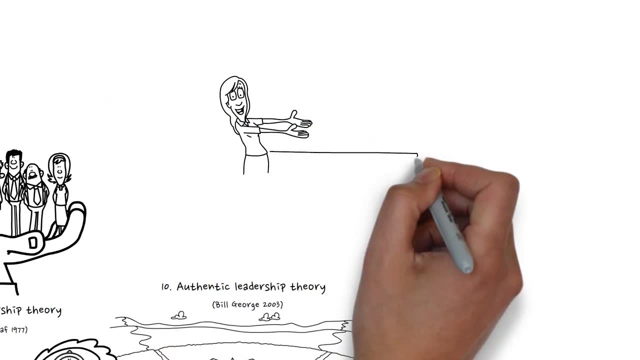 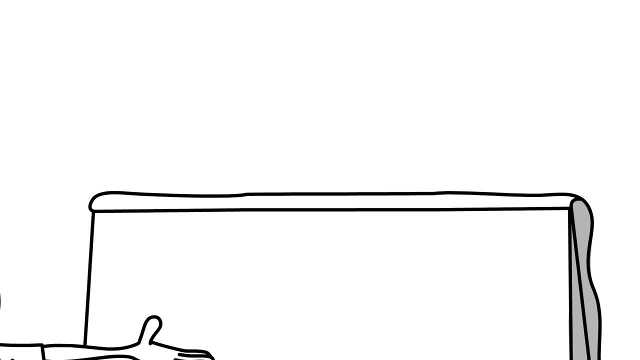 corporate management, such as the fraudulent behaviour that led to the fall of energy giant Enron. George advocated for leaders of purpose, values and integrity, rather than those motivated by greed and power. George's academic colleagues Bruce Avoglio and William Gardner then developed models. 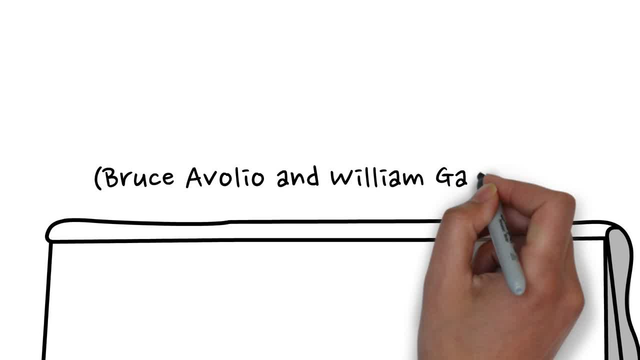 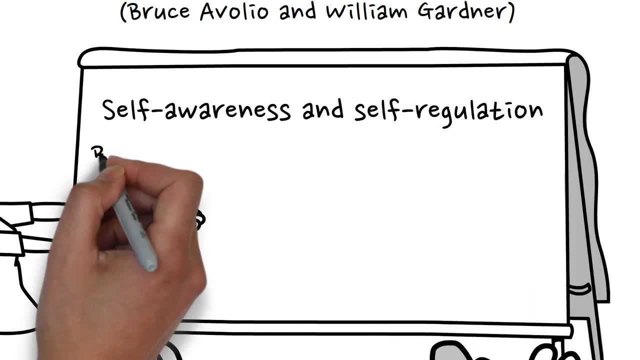 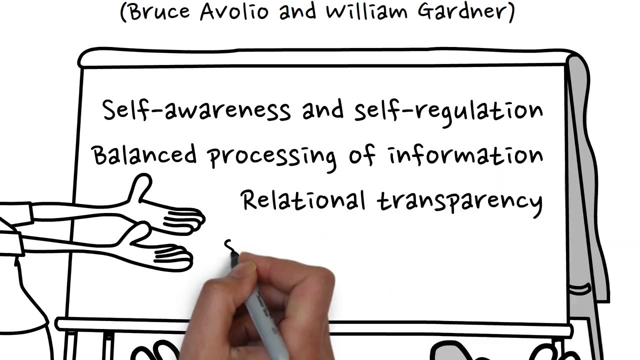 around this concept, identifying the key behaviours or traits of an authentic leader. These included self-awareness and self-regulation, balanced processing of information, relational transparency and a strong sense of morality. So that is a very quick introduction to some of the key leadership schools, theories and models. 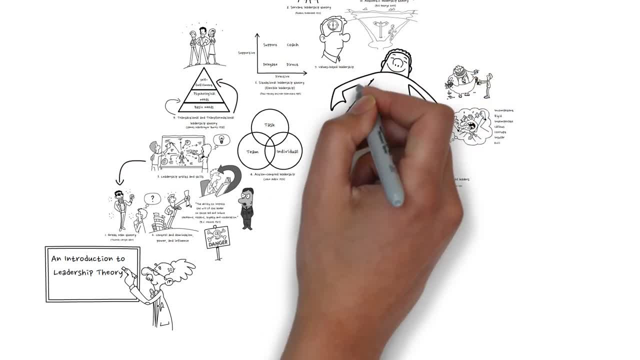 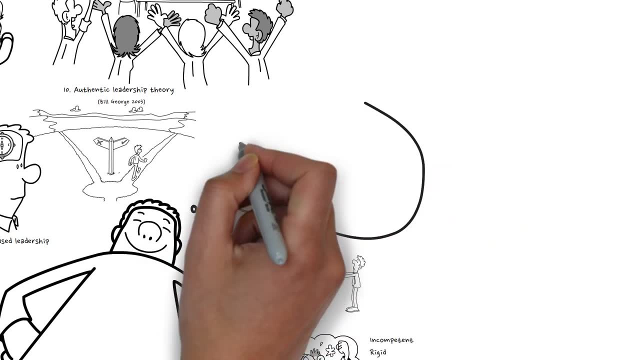 Theory can be a little dry, but understanding these models is important. They help to give us language and concepts. They help us reflect on our own leadership experience and the conduct of others. They give us tools to help and to use in our own leadership practice. And they also act. 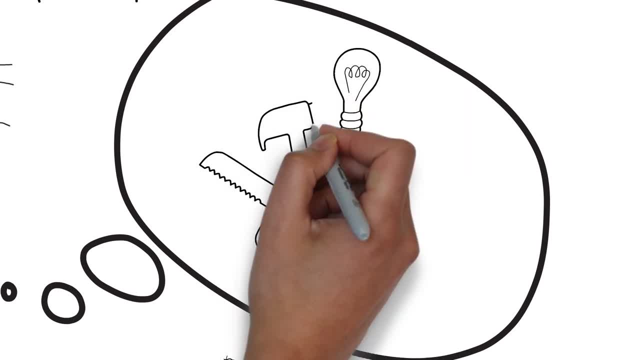 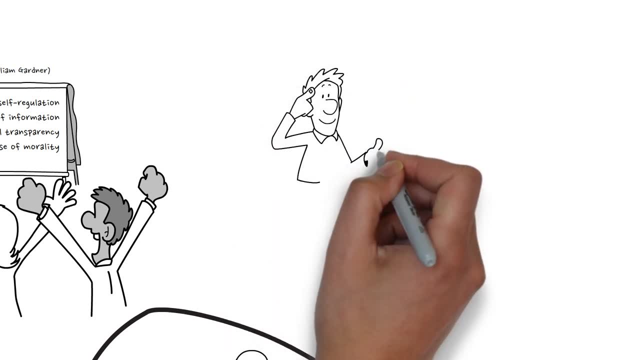 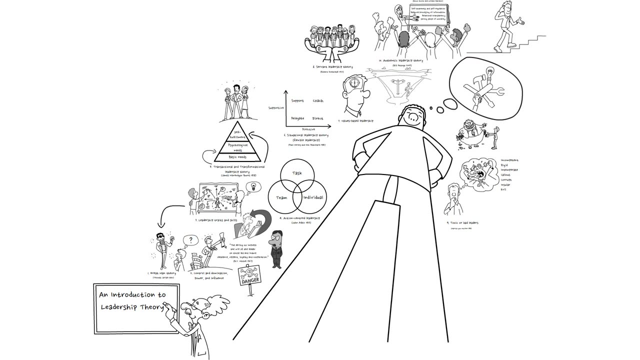 as signposts of ways that we can help to develop and grow other leaders. And you can start now. Take a few minutes to reflect Which of the leadership theories are most intriguing to you. What does this model reveal about your own leadership? Which tool could you apply in the interactions that you have today?